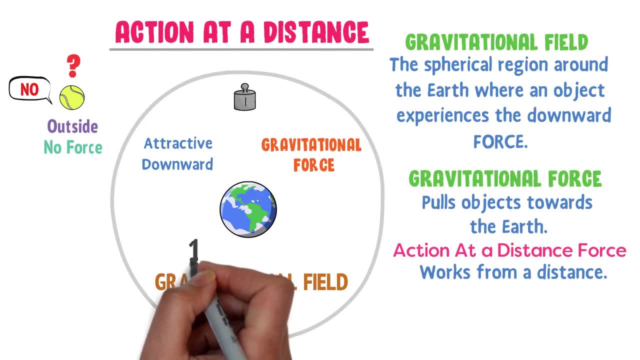 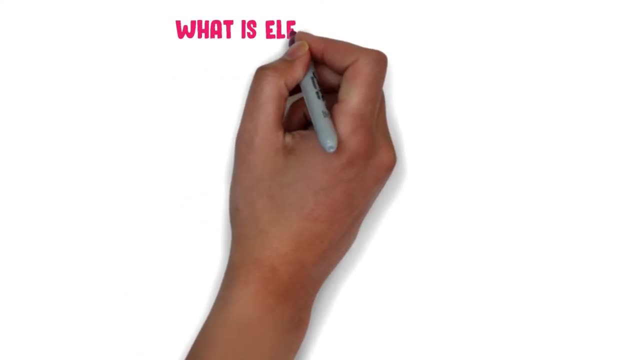 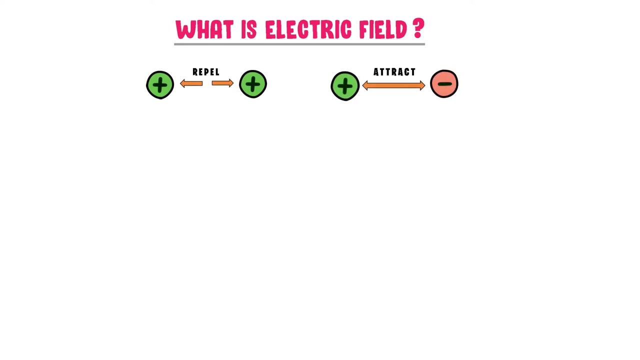 we learn two fundamental concepts. Firstly, there is gravitational field around the earth. Secondly, we learn that an object present in a gravitational field of the earth experiences the downward force of gravity. Now, what is electric field? Well, we know that like charges repel and unlike charges attract. But how? the like charges repel and unlike charges attract. 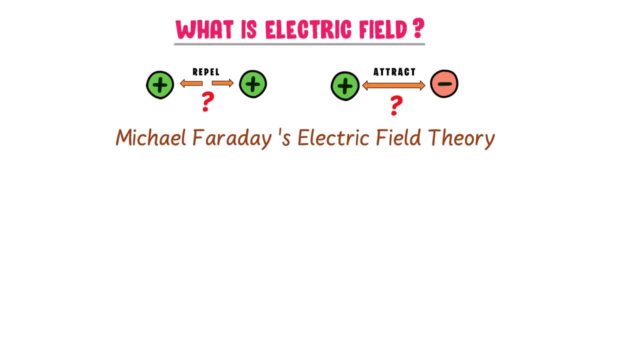 Well, it was Michael Feroldi who firstly put forward the theory of electric field. Now let's consider two big charges: positive and negative. According to Michael Feroldi, there is electric field around this positive charge, and there is also electric field around 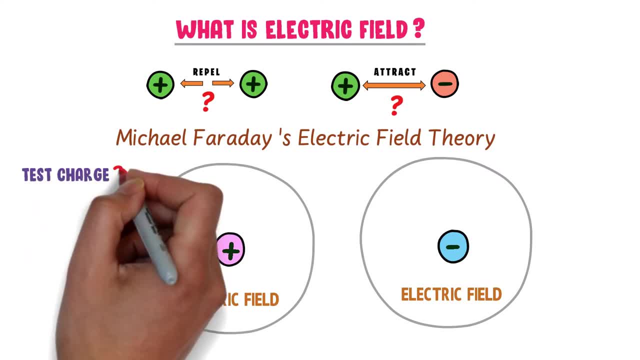 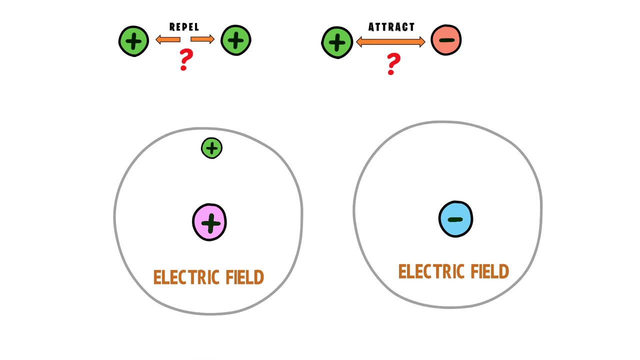 this negative charge. Now, what is a test charge? A test charge is a small positive charge. It has negligible effect on the electric field of other charges. For instance, it will not distort the electric field of positive or negative charge. Now let's consider that I bring a test charge. 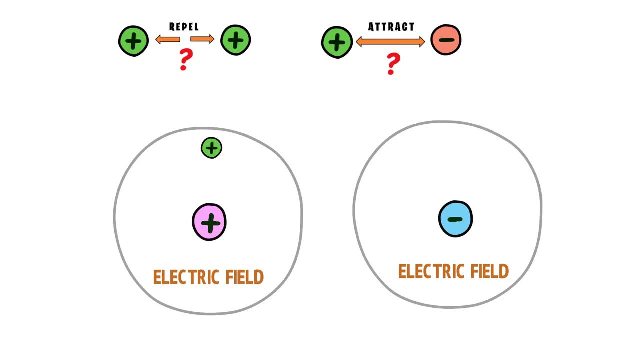 inside the electric field of positive charge and negative charge. This test charge experiences the force of electric field of positive charge, and this test charge also experiences the force of electric field of negative charge. So here test charge experiences repulsive force, and here test charge experiences attractive force. Now, if a test charge is present, 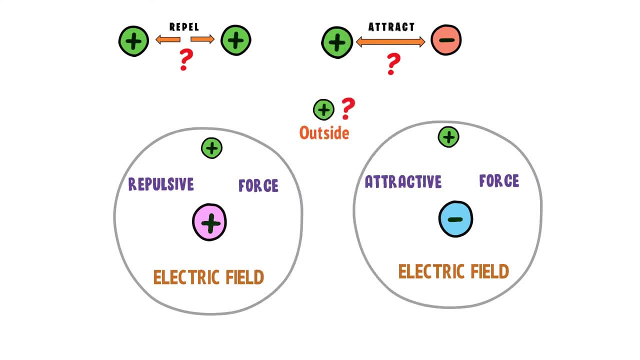 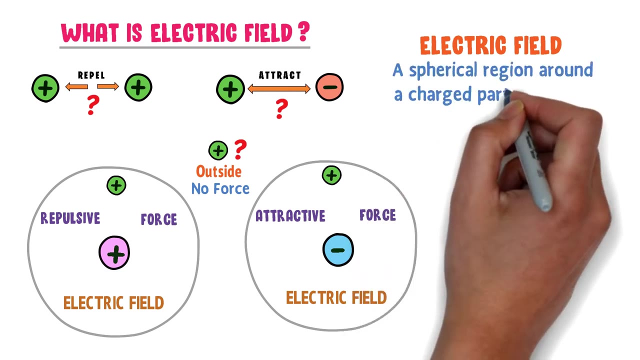 outside the electric field. does it experience repulsive force or negative force? Well, experiences any repulsive or attractive force? The answer is no, because it is outside the spherical region. Thus we define electric field as a spherical region around a charged particle. 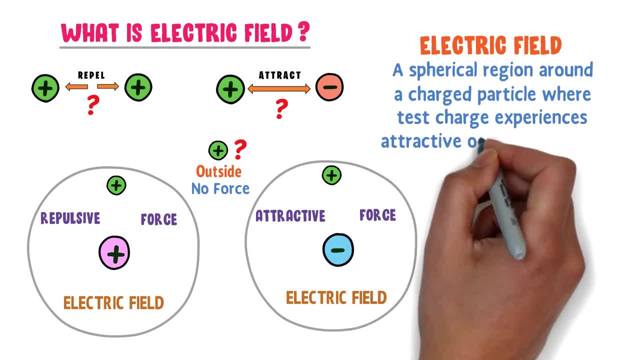 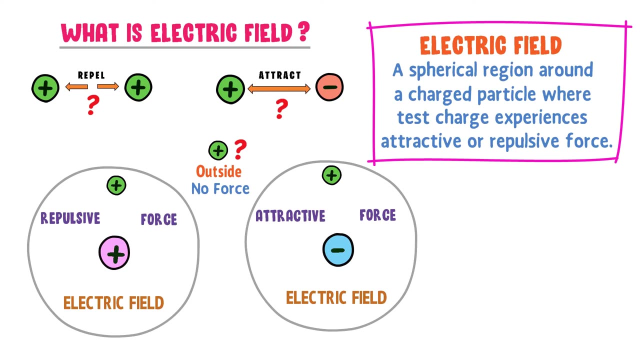 where test charge experiences attractive or repulsive force is called electric field. Let me repeat it: A spherical region around a charged particle where test charge experiences attractive force or repulsive force is called electric field. Note it down that the attractive or repulsive force in electric field is called electrostatic force. Thus we learn two important 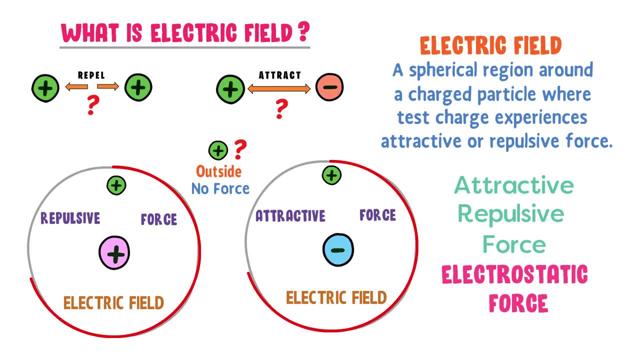 concepts. Firstly, there is a spherical region around any charged particle where test charge experiences attractive or repulsive force. Secondly, there is a spherical region around any charged particle where test charge experiences attractive or repulsive force. Secondly, this attractive or repulsive force within electric field is called electrostatic force. 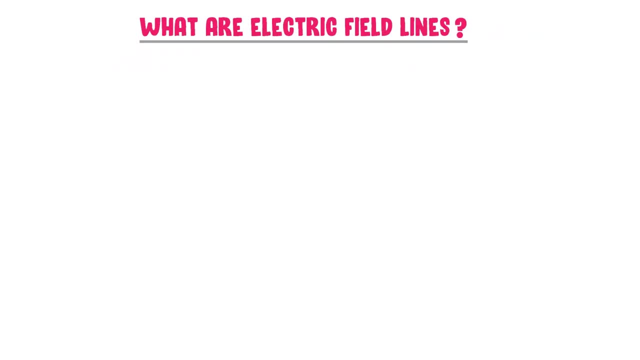 Now, what are electric field lines? Well, consider two charges, positive and negative. As we learnt in the previous slide that if I bring a test charge near a particle, it will have a positive charge. there will be repulsion between them and test charge will. 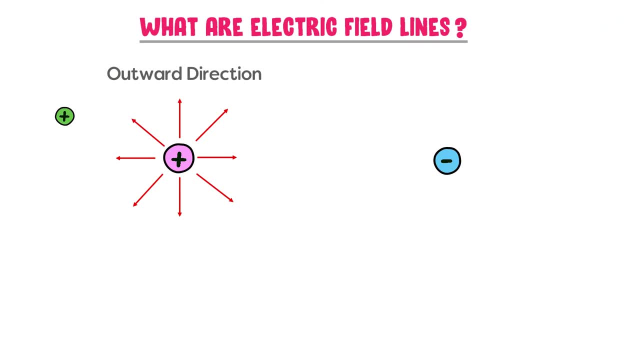 move away in outward direction. So we say that electric field lines originate on positive charges. Secondly, if I bring a test charge near a negative charge, there will be attraction between them. So we say that electric lines terminate on negative charges. The imaginary 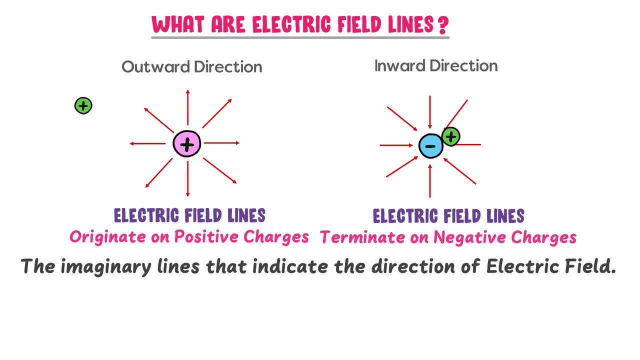 lines That indicates the direction of electric field is called electric field lines. Secondly, we can also define electric field lines as a path along which a positive test charge would move, if it is freely allowed to do so. Let me repeat it: A path along which a positive test charge would move if it is freely allowed to do so. 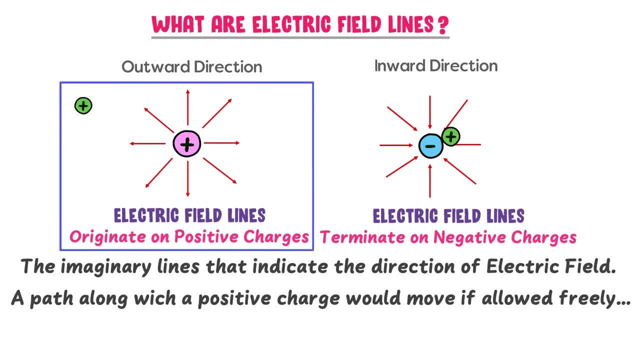 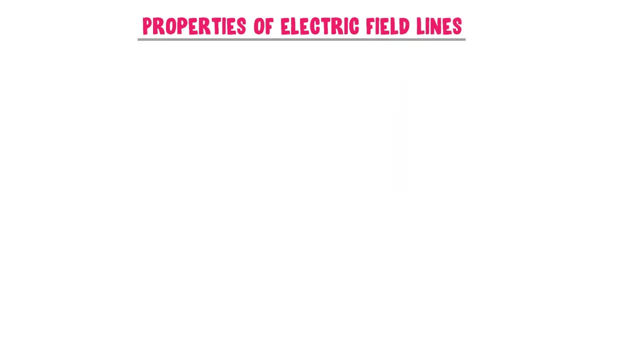 Thus, remember that electric field lines originate outwards on positive charges and terminate inward on negative charges. Finally, let me teach you the properties of electric field lines. Well, electric field lines are imaginary. Secondly, they never intersect each other. Thirdly, when the electric field is stronger, 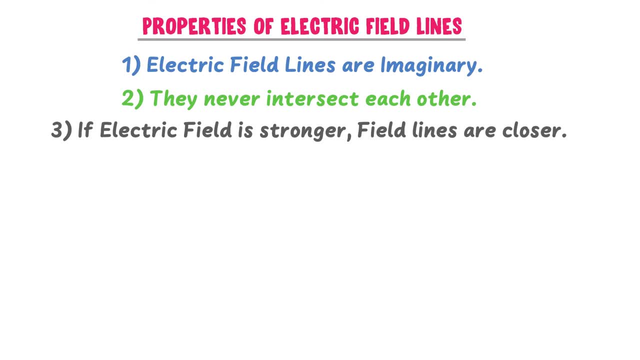 the field lines are not intersected. For example, at point A electric lines are closer, and here electric field is strong, While at point B field lines are away and here electric field is weak. Fourthly, electric field lines are perpendicular to the surface charge.